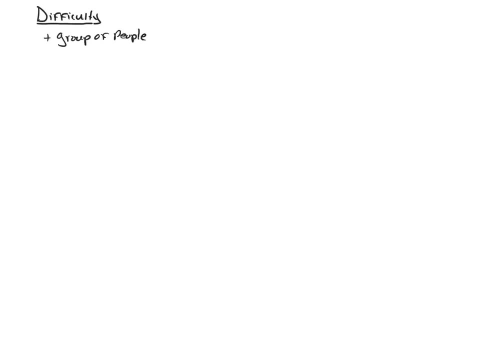 encountered a specific item, then the difficulty that we calculate from those five people. there's going to be significantly more uncertainty surrounding that difficulty or surrounding how confident we are that that difficulty is a good representation for a large population, versus a situation where perhaps 100%. 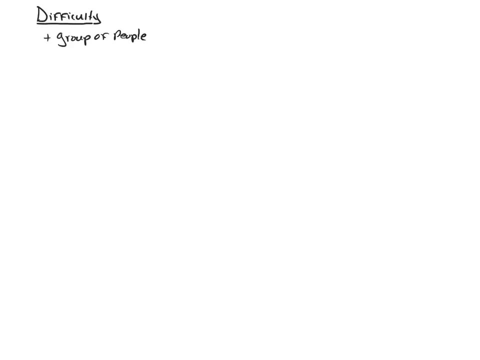 people have been exposed to an item And the difficulty that we get when 100 people have been exposed to an item. in general there's going to be a higher degree of confidence that that difficulty is more reliable than when only five people have taken it. So again, groups of people. 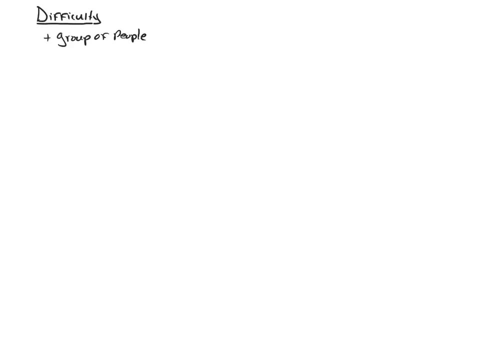 are a very important concept when it comes to difficulty And, in fact, it's very important when it comes to virtually all components of item analysis. Things just get better and better, And they should get better and better and better as more and more people take our exams and we make. 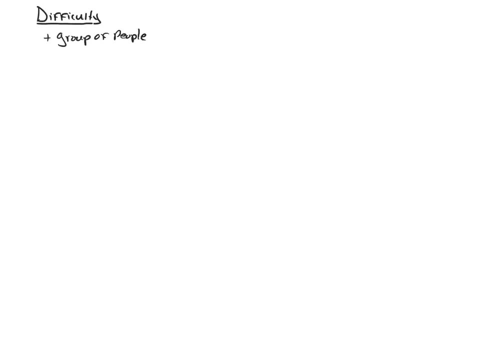 changes and we really zero in on the best questions that we can get. Okay, so how do we identify the difficulty of each item? Well, the difficulty- calculating difficulty is actually very easy. All right, this is the difficulty. Some people may call this the difficulty index or the index of 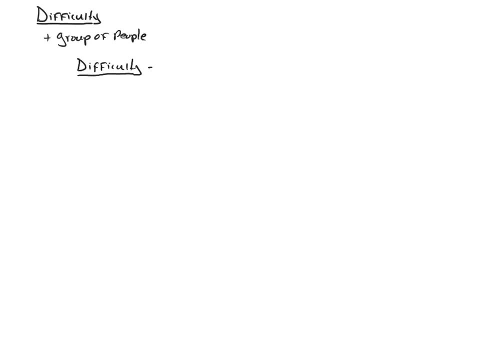 difficulty. We'll just call it the difficulty, And difficulty equals the number of students or candidates who got the answer correct- okay, who were correct All right- divided by the total number of students who were exposed to the item. So the total number of students who were exposed to that item- So, for example, let's say that I have 100- 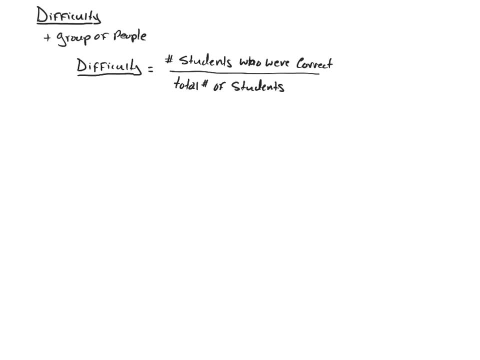 students that are that have taken a test? All right, So that's my total. All right is 100 students. All right, 100 students have taken that test And out of those 100 students, 48 students correctly answered that question. All right, So to calculate the difficulty, it's very easy. 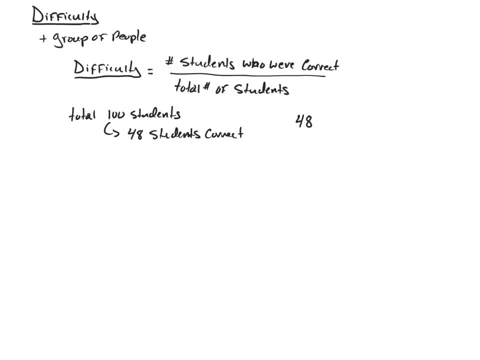 Right. So the number of students who are correct, there were 48 correct students divided by the total number, that's 100.. So 48 divided by 100 gives us a difficulty of 0.48.. All right, And that's on one item. 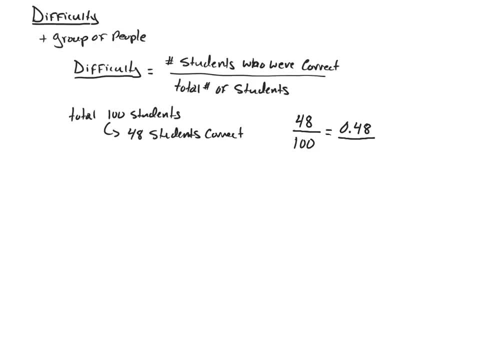 so what we'd have to do to find the difficulty is we will find the difficulty of the entire exam- is we need to do that with every item so that maybe that was item one and we got a difficulty of zero, point four, eight and then maybe item two. 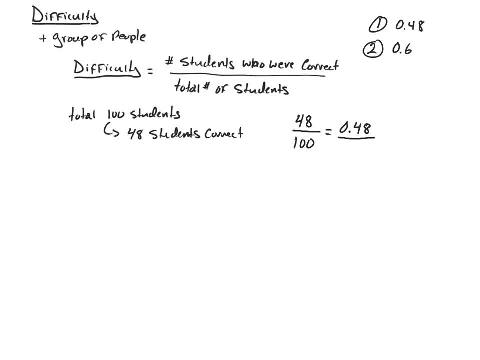 we got a difficulty of zero: point six, six and then item three. we got a difficulty of zero: point two, one and then item four. we got a difficulty of zero: point nine, eight, okay, all right, so I just threw some examples of item difficulty there, and then we'll go ahead and talk about what does that mean? okay? 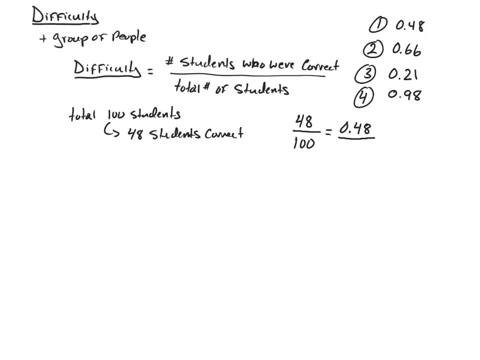 in general. well, when we think about it- I'll draw a little little line graph here, if you will, all right. and difficulty goes from zero to one, all right. and then we have zero, point five in the middle, all right, and so zero. if I get zero for my item, difficulty that means. 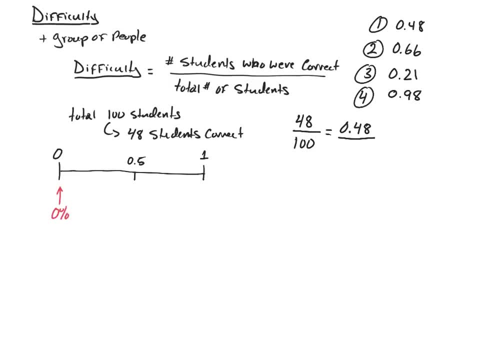 zero percent of the students who encountered that item were correct. so basically, everybody got that question right wrong, okay, and that typically represents a highly difficult. that represents a very difficult question and then one, okay, a difficulty of one would mean that 100% of the students answered that item correctly. well, what does that? 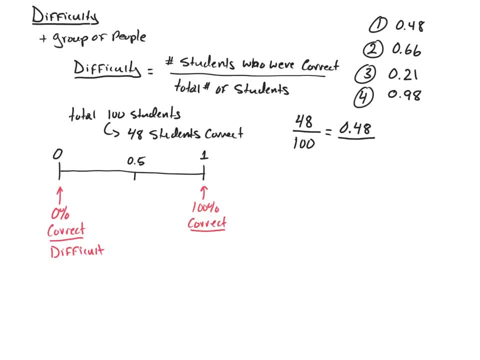 mean. well, that that's a ridiculously easy item, right, so that's very easy, and so from zero up to one is ridiculously difficult to ridiculously easy with most of our questions. okay, when, when, when? looking at the statistics, we would want most of our questions to more or less be in this area. right here, we want them to more, or 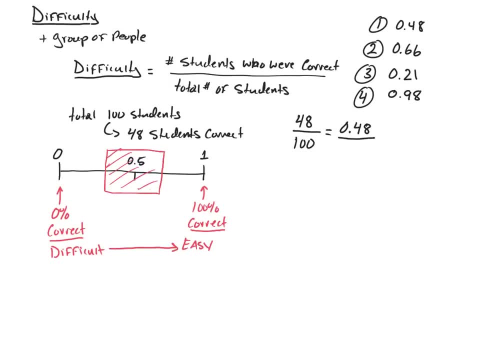 less Center around a zero point five and so for in general. okay, this is just a just a general rule of thumb. When we look at difficulty, we typically look for a question that has a difficulty of about 0.4 to 0.6.. Okay, this is kind of an average starting point That. 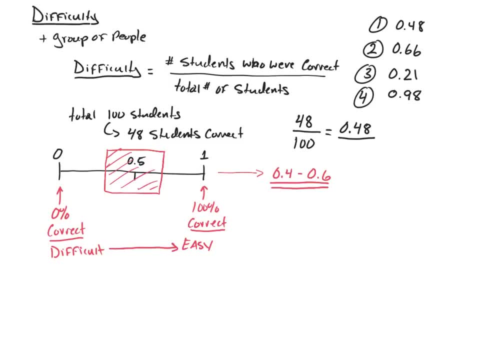 means 40 to 60% of the students that encounter this item will get this item correct And that kind of makes sense from a statistical standpoint when we look at a Gaussian distribution If we're wanting to have a good normal distribution right on our exam. you know you're going to see. 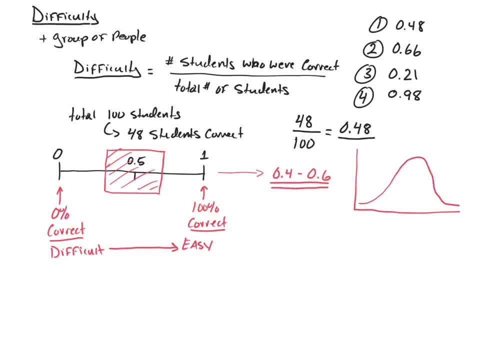 something like this on the individual items: Again, we're looking at individual items here, right? So you know this is, you know, 0.5, 0.6, 0.4,, right, And so you have a. 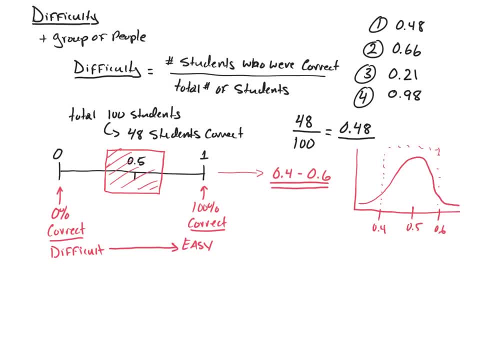 good. okay, you're representing a good chunk of your students here. okay, If you are shooting for a 0.4 to 0.6 with your outliers, okay, you have outliers here very, very difficult questions and you have your outliers here- very easy questions, Okay. so again, just a general rule. 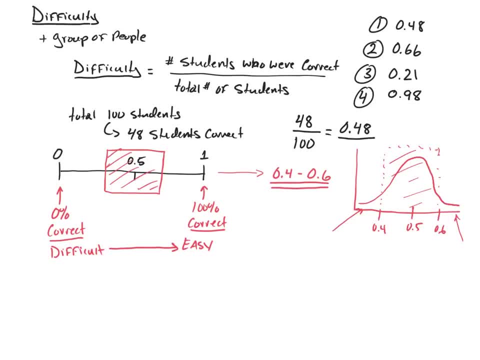 of thumb, And so we can kind of come down to some other general rules. And then, basically, if we have a difficulty, that's less than 0.3, these tend to be very difficult. These tend to be too difficult, All right. so less than 0.3 tend to be too difficult, All right, and greater. 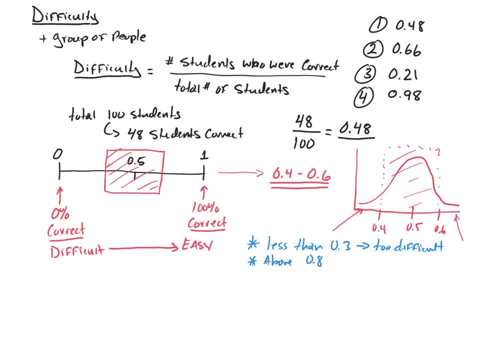 than or above 0.8 tend to be questions that are too difficult, All right. so if we have questions in our exam that have difficulties that lie outside of this range- either higher or lower than this range- we want to be rather judicious about having those. 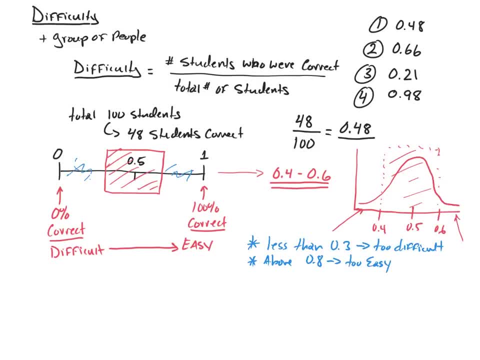 questions in our exam. We certainly would want to include some difficult and some easy questions, but we would want the majority of our questions to be in that 0.4 to 0.6 range. These very hard and very easy questions tend to be less reliable. All right, these tend to be less. 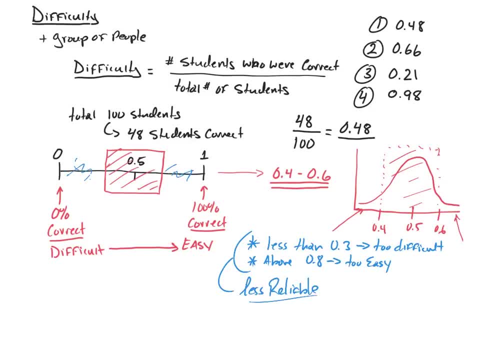 reliable for our exam. However, we would still want to include some of each to appeal to a broad range of students. So when we go here: okay, this question here has a difficulty of 0.48.. Okay, which lies on the lower end of the general range that we use. So these are questions at about. 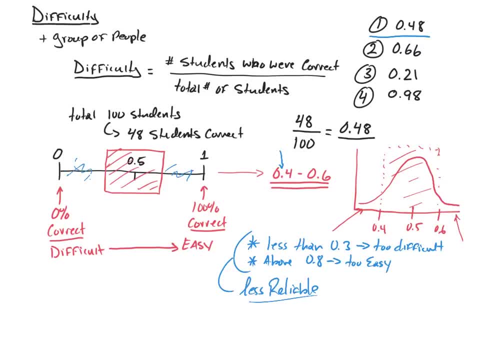 48% of the entire of the students that encountered that item got correct. Okay, so that's a little more. on the difficult end of the range, 0.66 is just a little higher than the 60%, So 66% of the students that encountered this question got it correct, So it's a little. 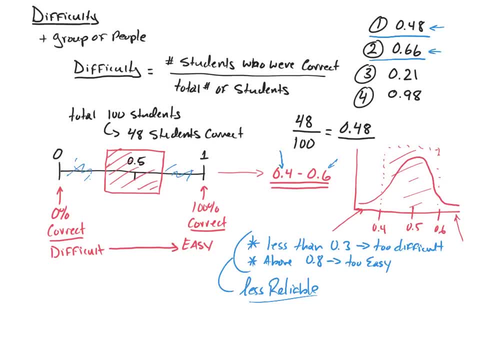 easier end of the range, a little outside of the range. 0.21,, however, is a very difficult question and only 21% of all the students got that question correct. And then 0.98 is a very easy question. 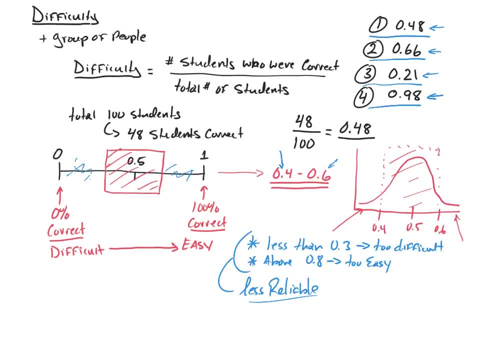 and that is 98% of the students got that question correct. Okay, so that's how we would, how we calculate difficulty, But that's not the entire 9 against 15 Story. The next thing that we need to do is, once we find a question and we recognize 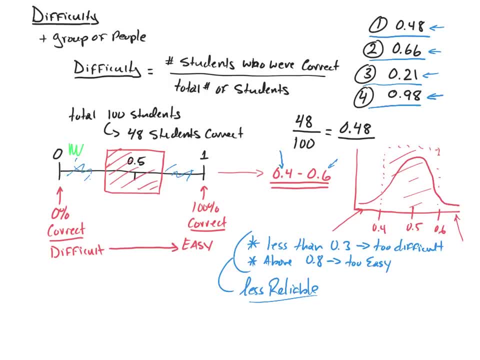 that a question is either more difficult than it needs to be or less difficult than we want it. okay, we need to ask ourselves: why Is it too difficult or too easy? Okay, and there are some very basic and some more nuanced reasons why that may be the answer. Okay, and that comes down.